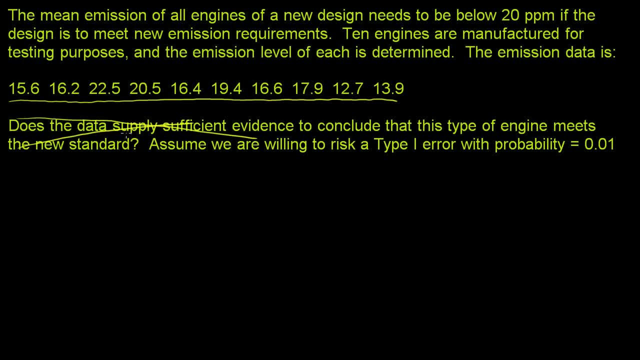 confidence interval for the actual mean emission for this new engine design. So we want to find a 95% confidence interval And, as you can imagine, because we only have 10 samples right here, we're going to want to use a t-distribution. 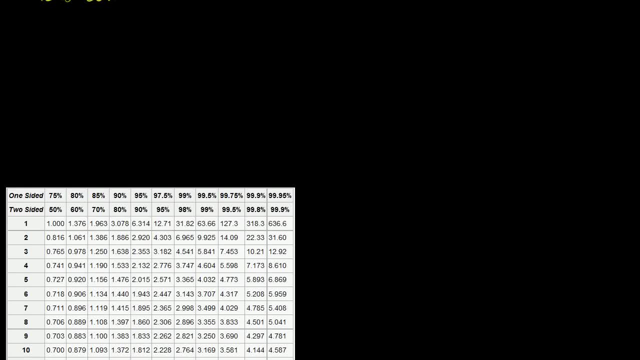 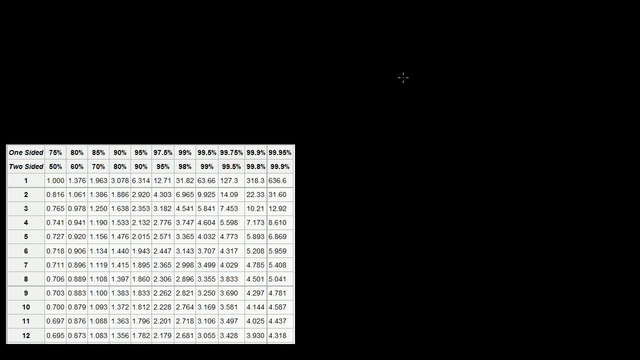 And right down here I have a t-table And we want a 95% confidence interval. So we want to think about the range of t-values that 95, or the range of t-values that 95, or the range of t-values that 95,. 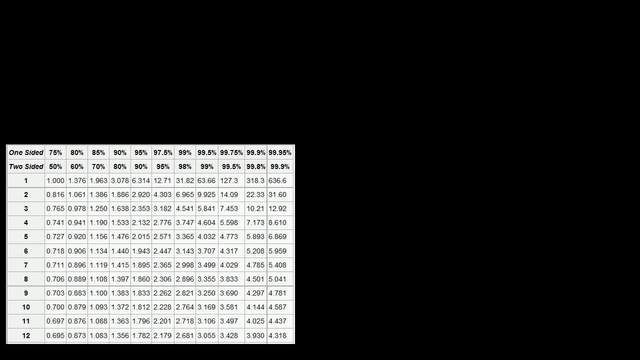 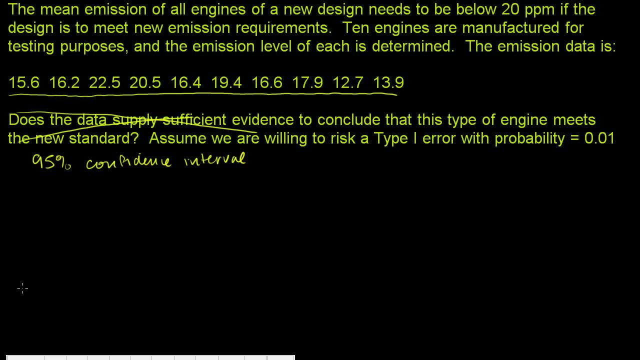 is the range that 95% of t-values will fall under. So let's think about it this way. So let me draw a t-distribution. Let me draw a t-distribution right over here, So a t-distribution looks very similar to a normal. 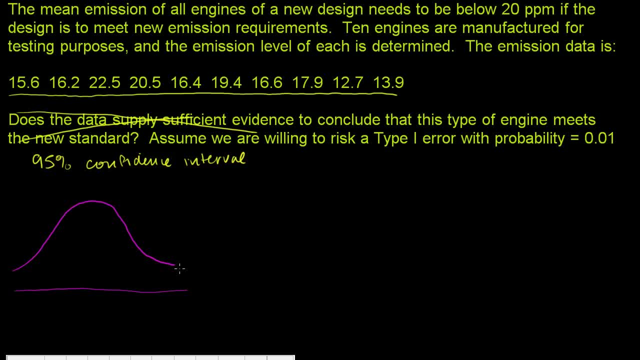 distribution, but it has fatter tails. It has fatter tails This end, and this end will be fatter than in a normal distribution. And then we want to find an interval. So this is a normalized t-distribution. The mean is going to be 0.. 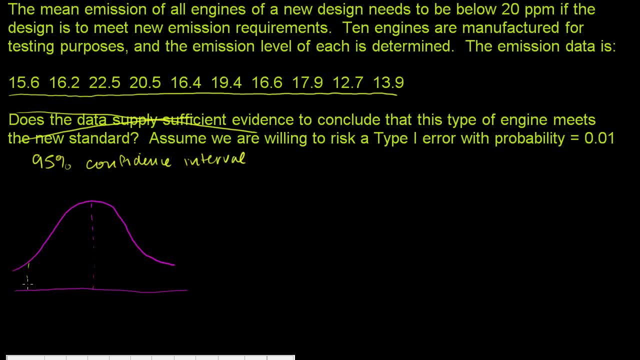 And we want to find an interval, And we want to find an interval of t-values between some negative value here and some positive value here that contains 95% of the probability. So this right here has to be 95% And to figure what these critical t-values are at this, 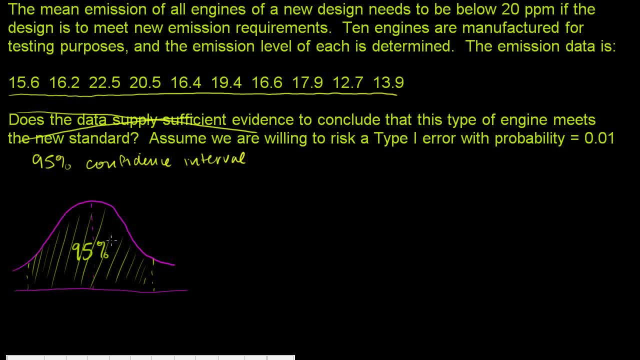 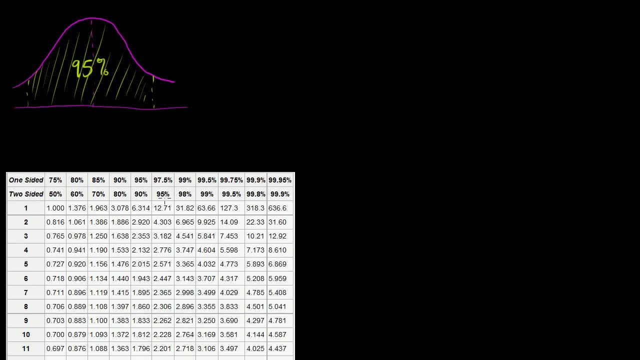 end and this end. we can just use a t-table And we're going to use the two-sided version of this because we're symmetric around the center. So you look at the two-sided. We want a 95% confidence interval, So we're going to look right over here. 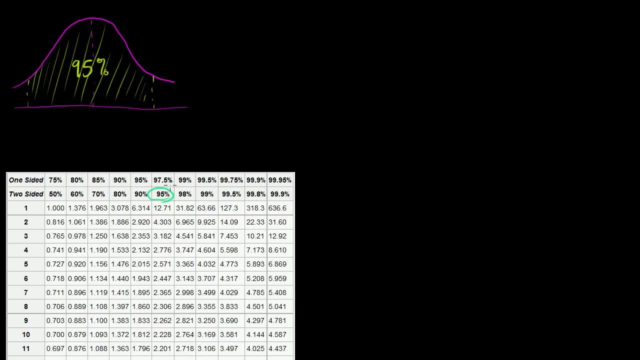 95% confidence interval. We have 10 data points, which means we have 9 degrees of freedom for our 10 data points. We just took 10 minus 1.. So if we look over here for a t-distribution with 9 degrees, 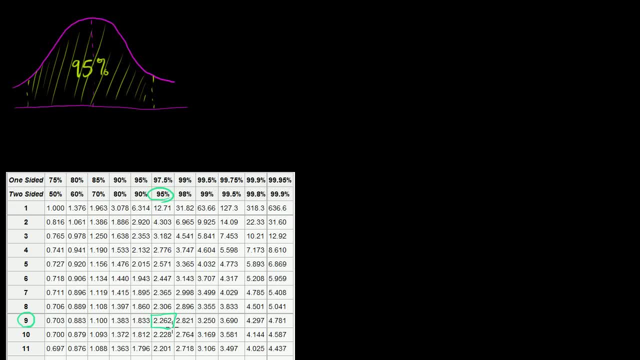 of freedom you're going to have, 95% of the probability is going to be contained within a t-value of. so the t-value is going to be between negative. So this value right here is going to be negative. This value right here is 2.262.. 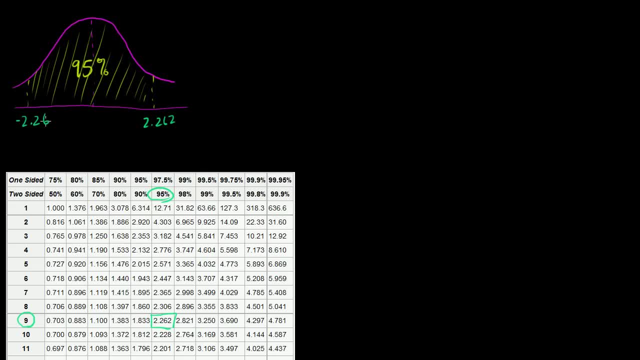 And this value right here is negative 2.262.. That's what this right here tells us: that if you contain all the values that are less than 2.262 away from the center of your t-distribution, you will contain 95% of the. 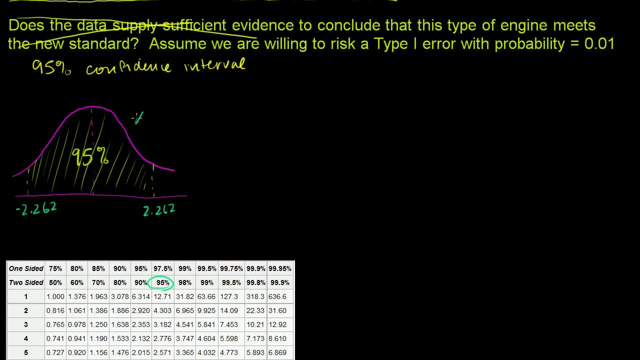 probability. So that is our t-distribution. right there, Let me make it very clear: This is our t-distribution. So if you randomly pick a t-value from this t-distribution, it has a 95% chance of being within this, far from the mean. 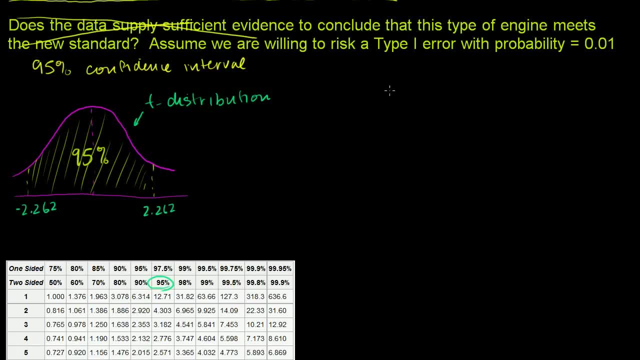 Or maybe we should write it this way: If I pick a random t-value, if I take a random t-statistic, there's a 95% chance that a random t-statistic is going to be less than 2.262.. 2.262 and greater than negative 2.262.. 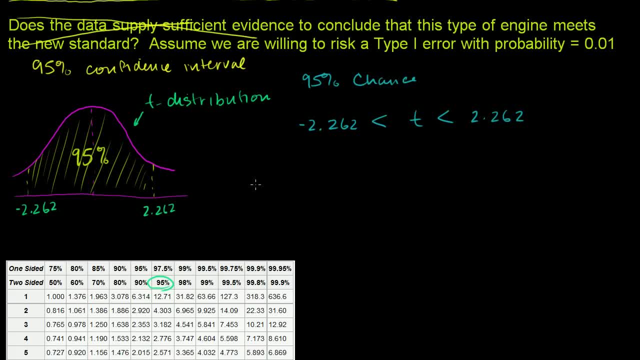 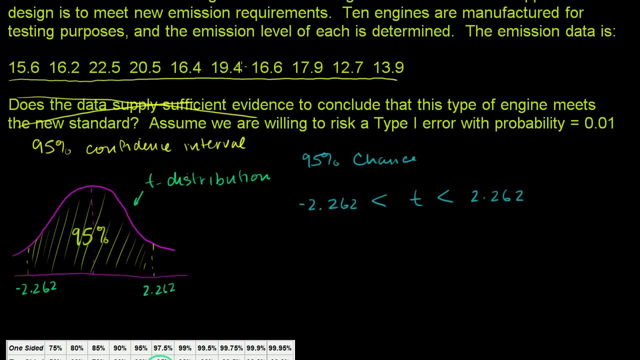 95% chance. Now, when we took this sample, we can also derive a random t-statistic from this. We have our sample mean and our sample standard deviation. Our sample mean here is 17.17.. 17.17.. 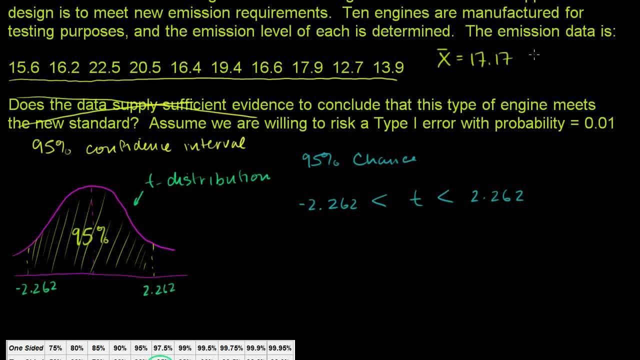 17.17., 17.17., 17.17., 17.17., 17.17.. Figure that out in the last video. Just add these up, Divide by 10. And our sample standard deviation here is 2.98.. 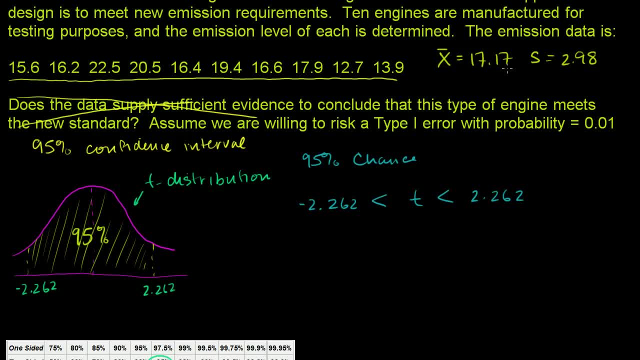 So the t-statistic that we can derive from this information right over here. so let me write it over here, The t-statistic that we can derive from this, And you can view this t-statistic as being a random sample from a t-distribution. 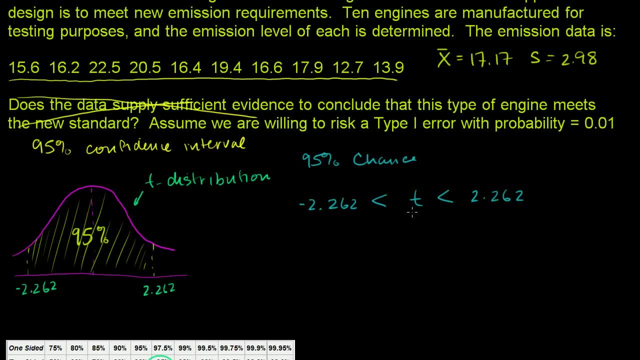 A t-distribution with 9 degrees of freedom. So the t-statistic that we can derive from that is going to be our mean 17.. 17.17 minus the true mean of our population, Or actually we say the true mean of our sampling distribution. 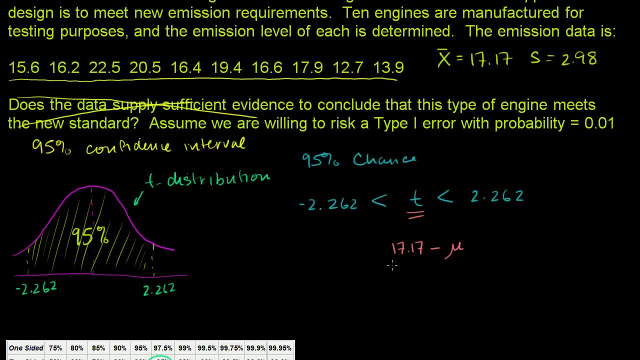 which is also going to be the same as the true mean of our population, That's, our population mean over there Divided by s, which is 2.98, over the square root of our number of samples. We've seen this multiple times. 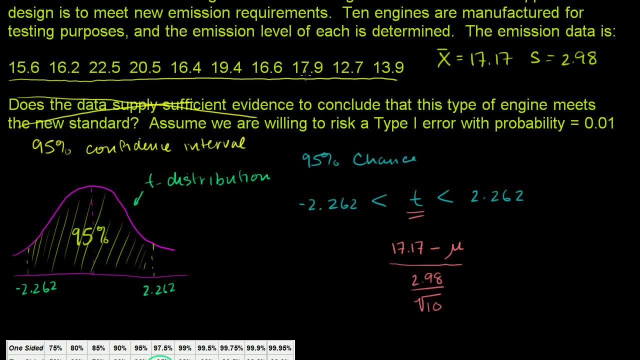 This right here is the t-statistic. So by taking this, Taking this sample, you can say that we've randomly sampled a t-statistic from this 9 degree of freedom t-distribution. So there's a 95% chance that this thing right over here. 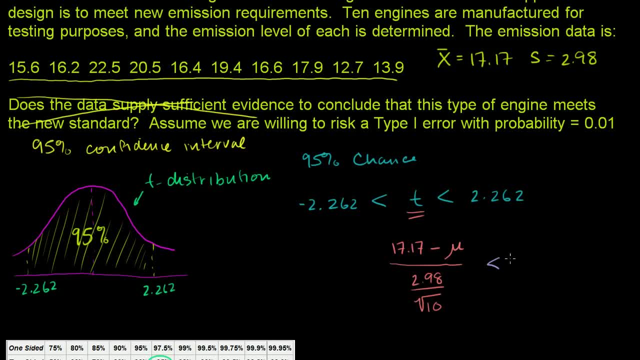 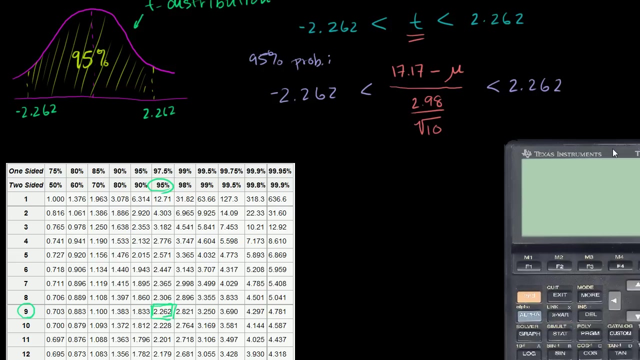 is going to be less than 2.262 and greater than negative 2.262.. So the 95% probability still applies to this. This right here. Now we just have to do some math, Calculate these things. Let me get my calculator out. 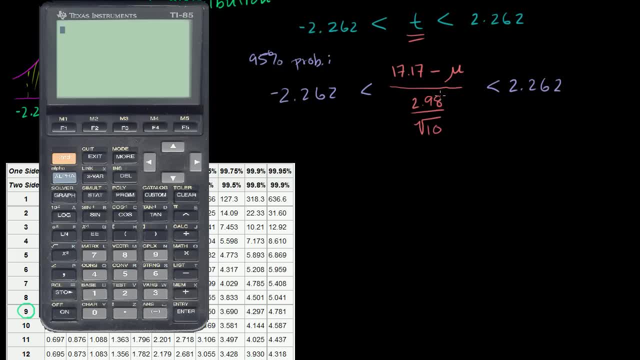 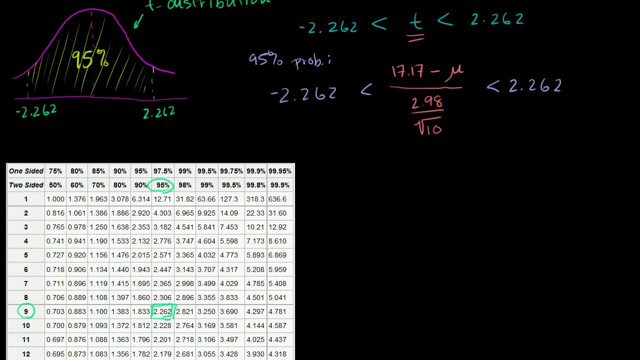 And get the calculator out, And so let me just calculate this denominator right over here. So we have 2.98 divided by the square root of 10.. So that's 0.9423.. So what I'm going to do is I'm going to multiply both sides of this equation. 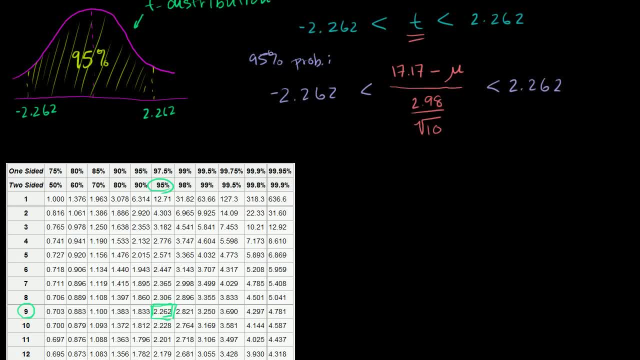 By this expression right over here. So if I do that, So let me just do that right over. So if I multiply this entire, This is really two equations, One or two inequalities. I should say That this quantity is greater than this quantity. 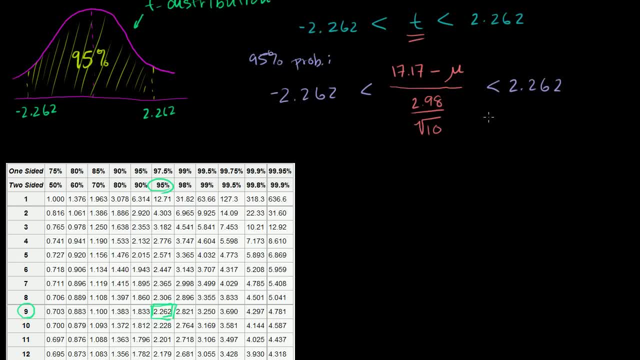 And that this quantity is greater than that quantity. But we can operate on all of them at the same time, This entire inequality. So what we want to do is multiply this entire inequality by this value right over here, And we just calculated that, that value. 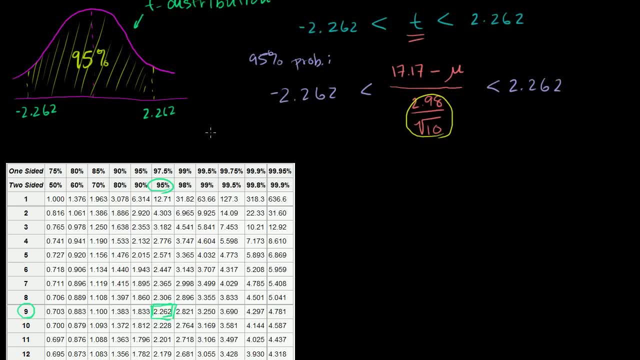 Let me write it over here: The 2.98.. I'll write it over here: 2.98 over the square root of 10 is equal to 0.942.. So if I multiply this entire inequality by 0.942.. 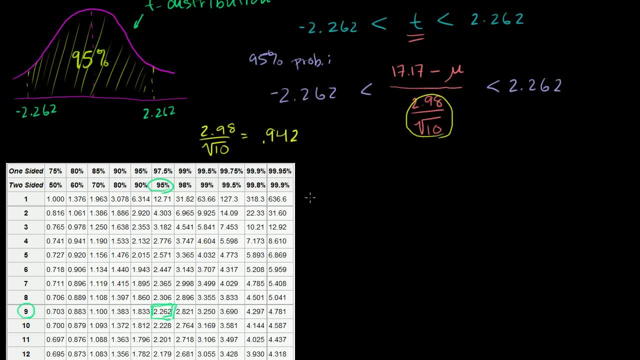 I get on this left hand side over here, I have negative 2.262 times 0.942.. And it's a positive number that we're multiplying The whole inequality by, So the inequality signs are still going to be in the same direction. 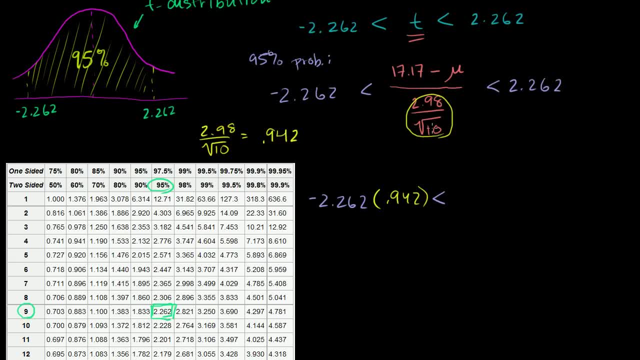 Is less than Well. we're multiplying this whole expression by the same expression in the denominator, So it'll cancel out. So we're just going to be less than 17.17 minus our population mean, Which is going to be less than 2.262 times, once again, 0.942.. Let me scroll down here a little bit, So that's going to be less than 2.262 times 0.942.. Let me scroll down here a little bit, So that's going to be less than 2.262 times, once again, 0.942.. 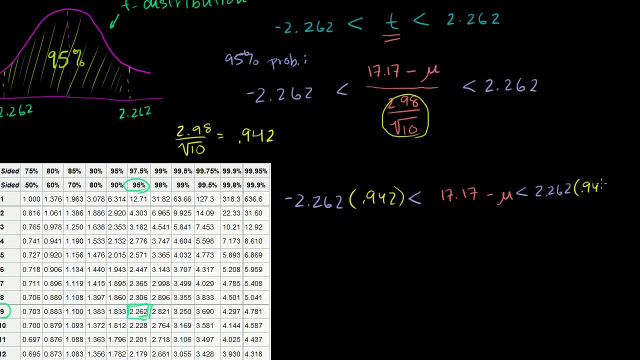 Let me scroll over to the right a little bit: 942.. Just be clear, I'm just multiplying all three sides of this inequality by this number right over here In the middle. this cancels out. So if I multiply I'll just write it right here. 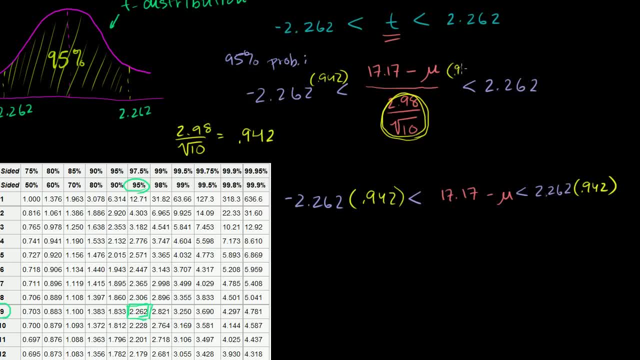 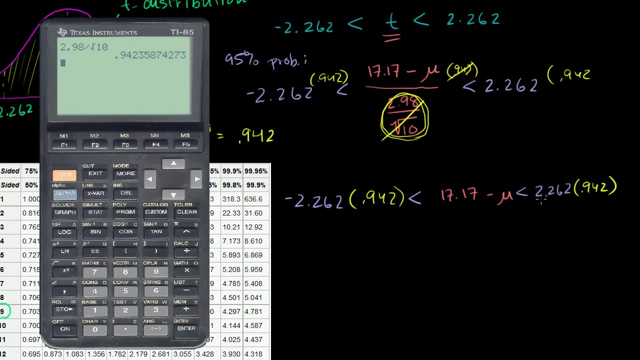 0.942.. 0.942. 0.942.. This and this is the same number, So that's why those cancel out. And now let's hit the calculator to figure out what these numbers are: 0.942.. 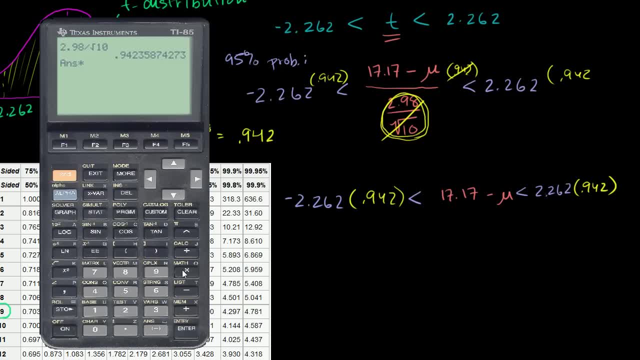 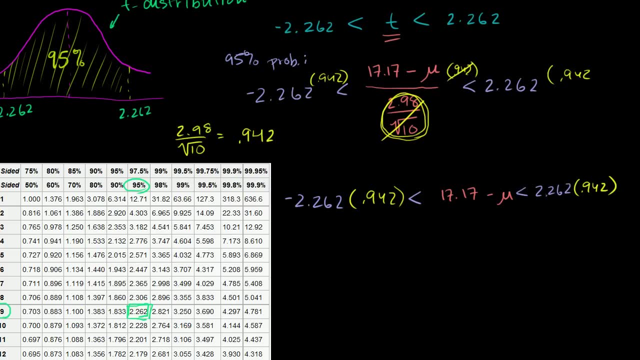 So we're going to say times is 2.13.. So this is going to be. So this number right over here on the right-hand side, This number on the right-hand side, is 2.13.. 2.13.. 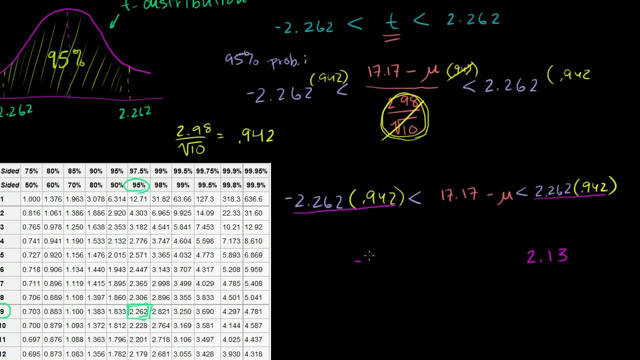 This number on the left is just a negative of that. So it's Negative: 2.13.. negative 2.13.. 0.942.. 2.13.. we still have our inequalities is going to be. 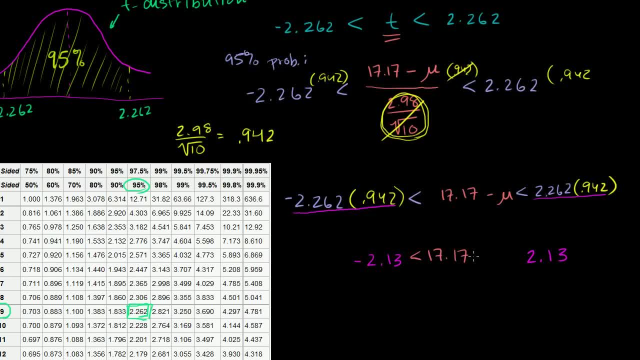 less than 17.17, minus the mean, which is less than 2.13.. Now what I want to do is I actually want to solve for this mean And I don't like that negative sign in the mean. I'd rather have this swapped around. 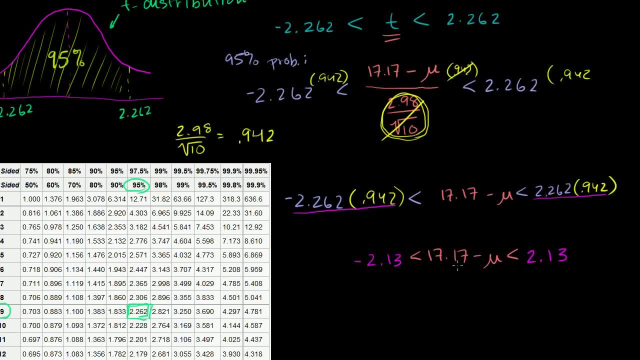 I'd rather have the mean minus 17.17.. So what I'm going to do is multiply this entire inequality by negative 1.. If you do that, if you multiply the entire thing times negative 1, this quantity right here, this: 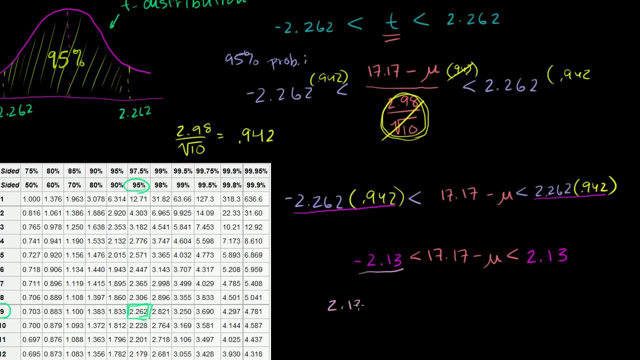 negative 2.13 will become a positive 2.13.. But since we are multiplying an inequality by a negative number, you have to swap the inequality sign. So this less than will become a greater than This negative mu will become a positive mu. 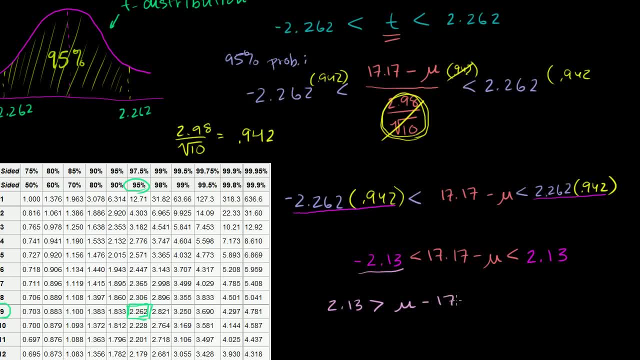 This positive 17.17 will become a negative 17.17.. We're going to have to swap this inequality sign as well, And this positive 2.13 will become a negative 2.13.. And we're almost there. We just want to solve for mu. 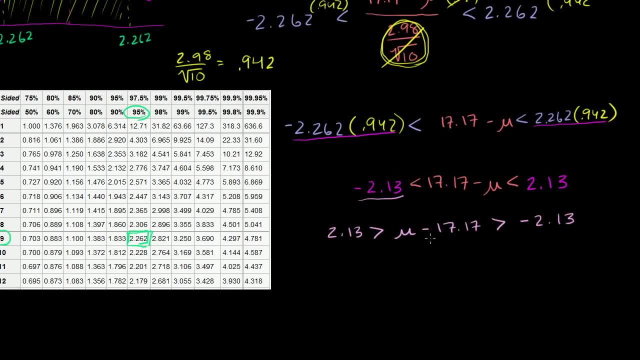 Have this inequality expressed in terms of mu. So what we can do is now just add 17.17 to all three sides of this inequality And we are left with 2.13 plus 17.17 is greater than mu, minus 17.17 plus 17.17 is just going to be mu, which. 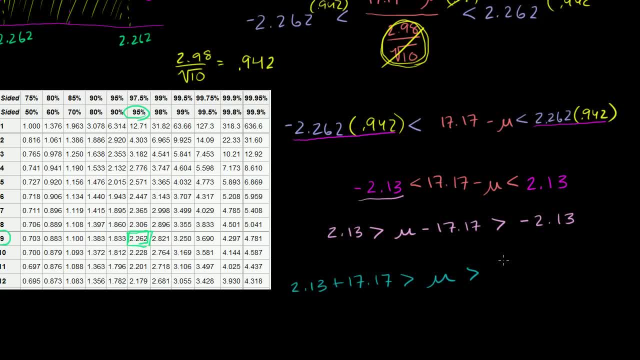 is greater than so. this is greater than mu, which is greater than negative 2.13.. 2.13 plus 17.17.. Or a more natural way to write it, since we actually have a bunch of greater than signs that this is actually the. 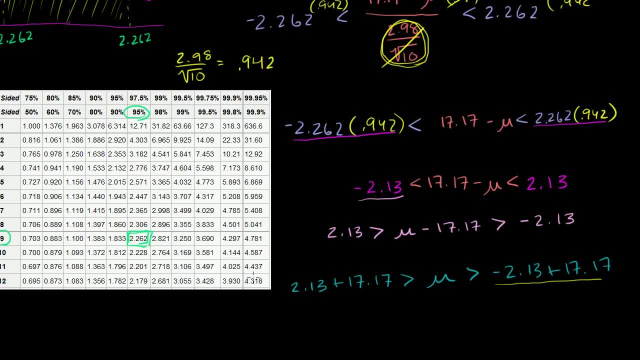 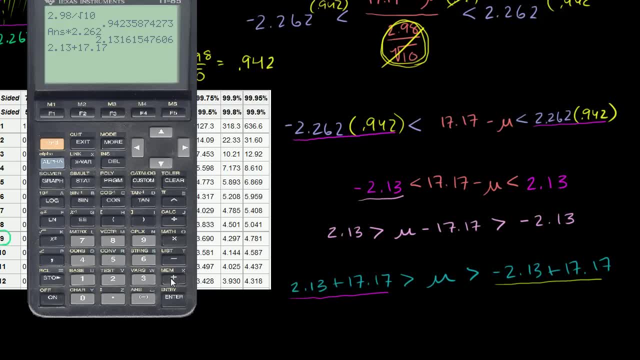 So we have 2.13 plus 17.17.. So we have 2.13 plus 17.17.. So that is the high end of our range. So that is 19.3.. So this value right over here, so this is 19.. 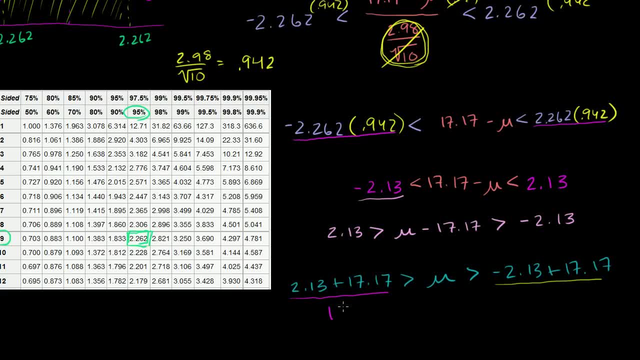 Let me do it in that same color. This value right here is 19.3, is going to be greater than mu, which is going to be greater than- And this is negative- 2.13 plus 17.17.. Or we could have. 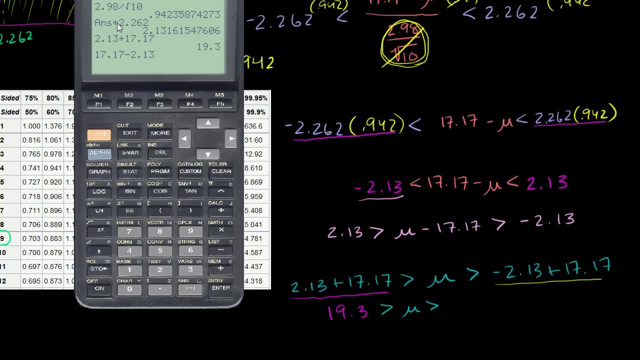 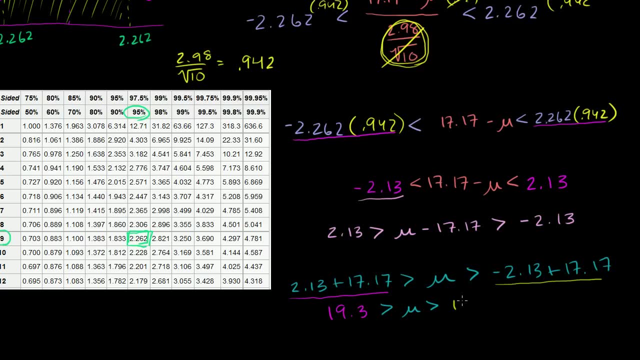 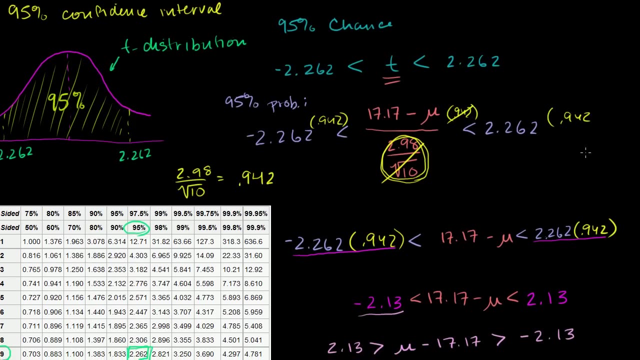 17.17 minus 2.13,, which gives us 15.04.. And remember the whole thing, all of this we started with. there was a 95% chance that a random t statistic will fall in this interval. 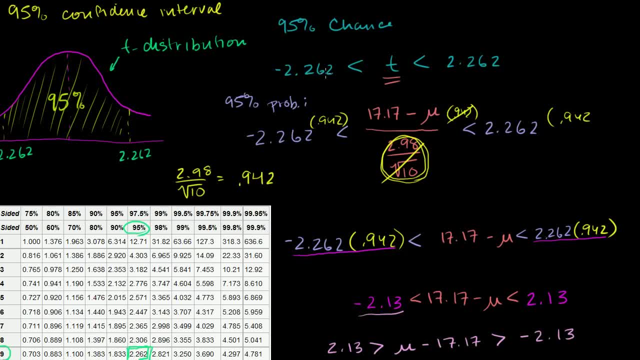 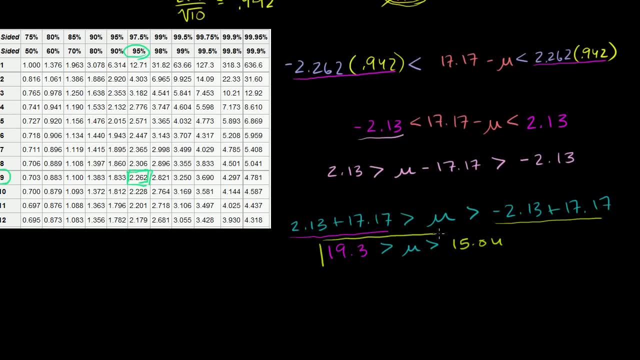 We had a random t statistic And all we did is a bunch of math. So there's a 95% chance that any of these steps are true, And so there's a 95% chance that this is true. There's a 95% chance that the true population mean, which is: 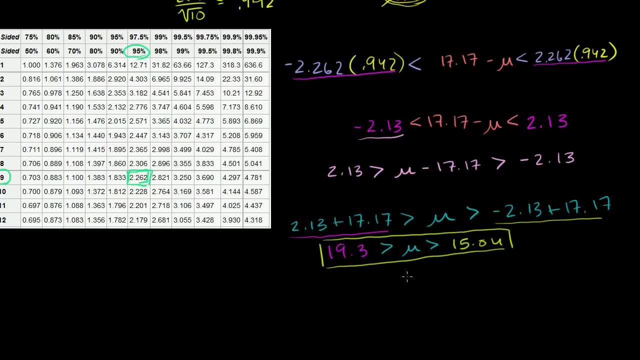 the same thing as the mean of the sampling distribution of the sample, mean there's a 95% chance, or we're confident that there's a 95% chance, that it will fall in this interval And we're done. 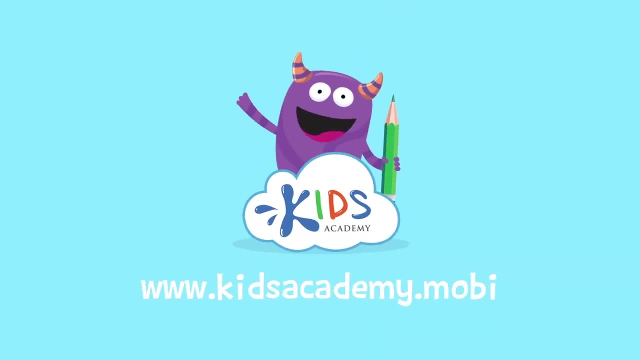 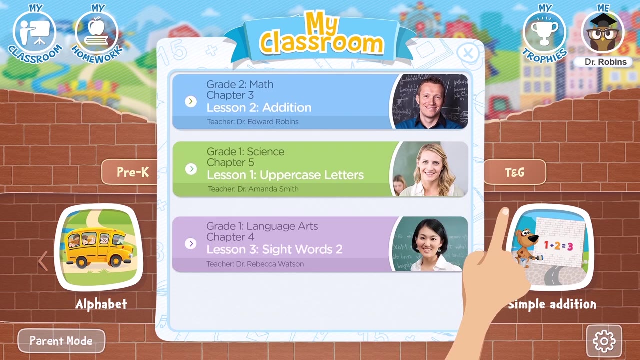 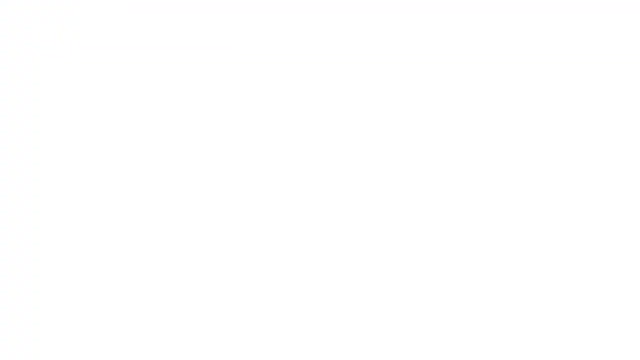 Welcome to kidsacademymobi. Hello everyone, Let's open the worksheet. Don't forget to like this video and subscribe to our channel. You can find the link to this app in the comments below, And today we're going to be looking at some 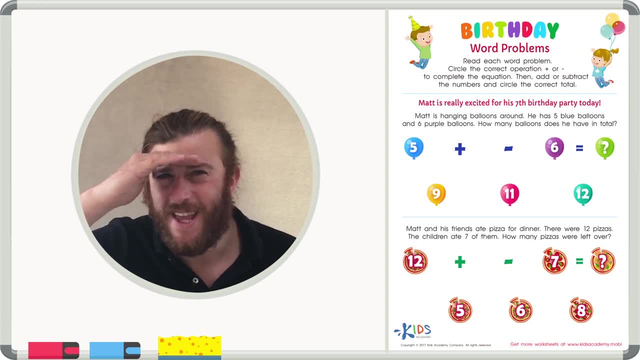 word problems. We're going to read the directions really carefully and read the word problems even more carefully. Let's get started right away. Birthday word problems. Read each word problem, Circle the correct operation to complete the equation, Then add or subtract the numbers and circle. 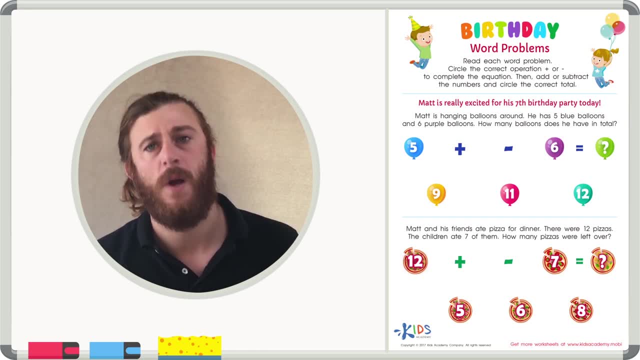 the correct total. So in this worksheet we're going to have to read the problems really carefully, figure out whether the problem is asking us to add or subtract, and then solve the problem. Let's get started right away. Matt is really excited for his seventh birthday party.